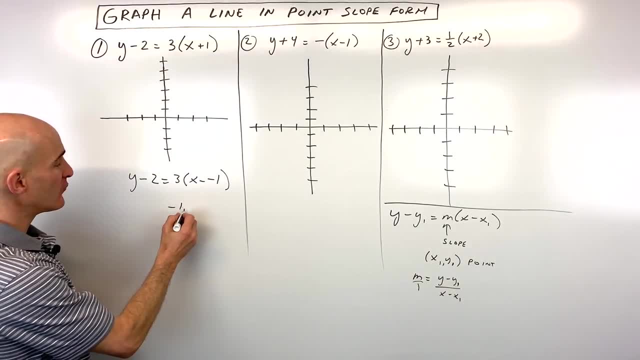 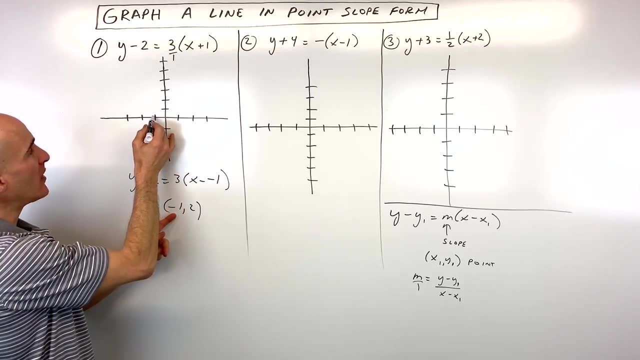 1, positive 2.. It's the opposite. So negative 1 comma 2, that's our point and our slope is 3, which is like 3 over 1.. So let's locate our point: negative 1 and the y coordinate is positive 2,. 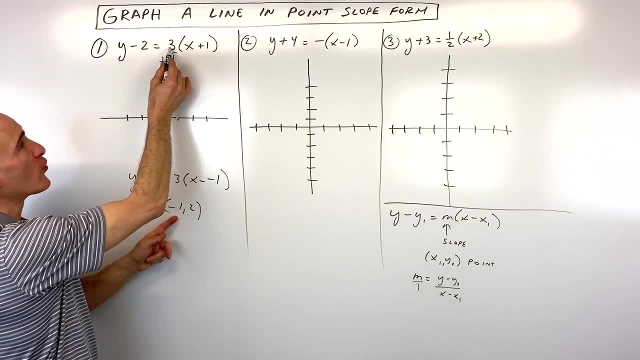 so up 2, and then, from this point now, what we're going to do is we're going to go rise 3 and run 1.. So the numerator is the rise, the vertical direction. we're going to go up 1,, 2,, 3, the run. 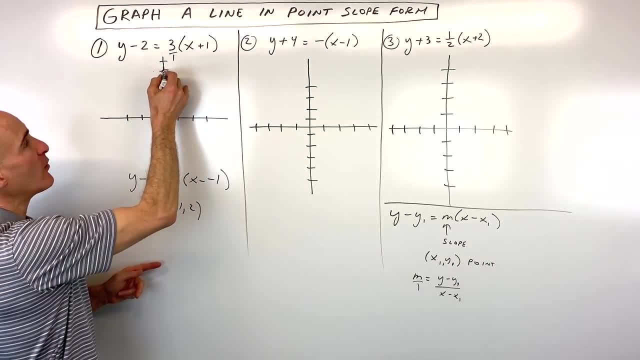 is the horizontal direction. it's positive: 1,, 2,, 3, and then we're going to go up 1,, 2,, 3, and then we're going to go down 1.. So I'm going right: 1, and we've got another point on our line. 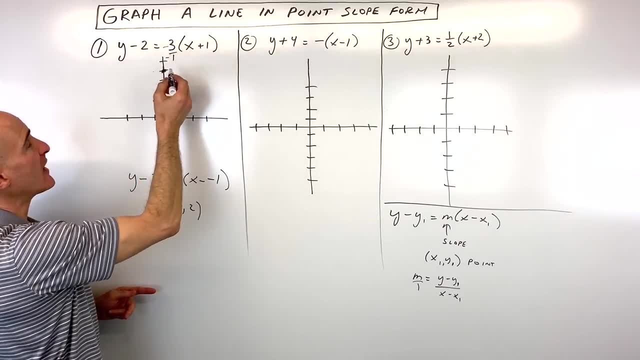 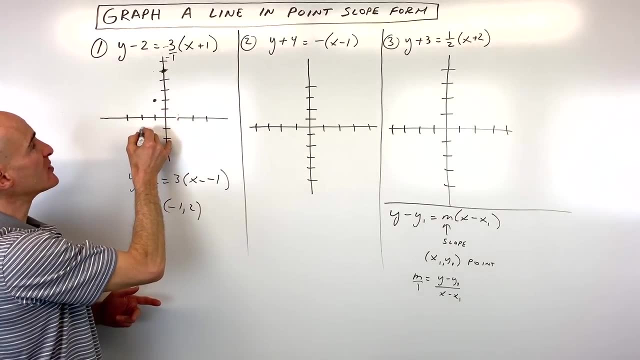 We can also reverse that. we can think of that as negative 3 over negative 1, because the two negatives cancel, And from this point we can go down 1, 2, 3 and then left 1.. You can see we're still getting the same line and you've got it. So let's do another example. 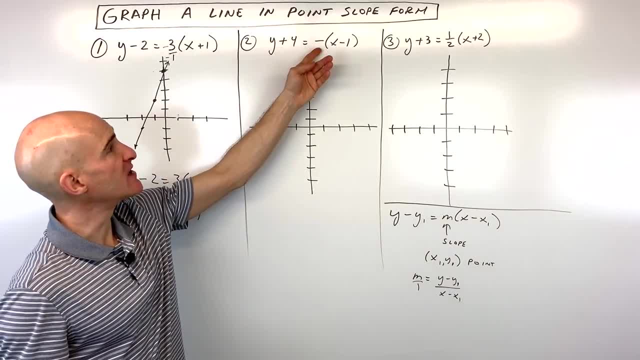 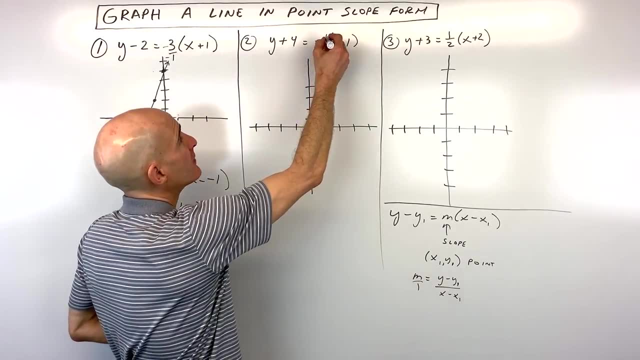 see if you can follow me here. So number 2: we've got. y plus 4 equals negative times x minus 1. So when you see this negative here, you can think of it as negative 1.. Okay, this because negative 1 times anything is going to be just like multiplying by a negative. 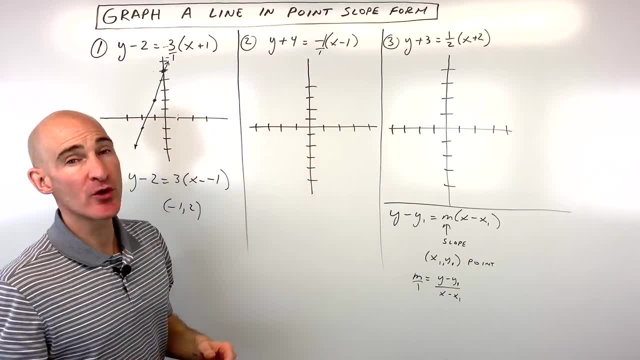 And you can write any number as a fraction by putting it over 1.. So when we do our slope, it's the rise over the run, The numerator is the rise, the vertical change, and the denominator is the run, That's the horizontal change. 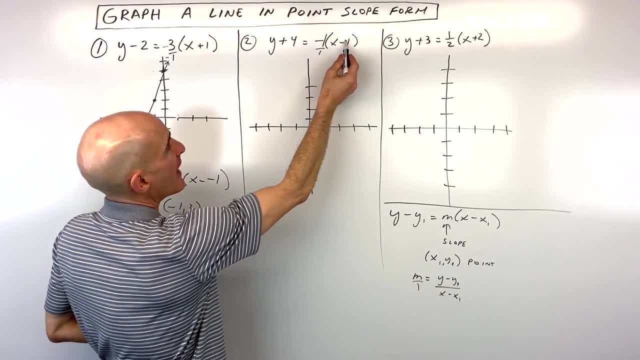 But you can see it's going through the point: positive 1.. Remember, the x-coordinate is a group of the x, The y-coordinate is a group of the y but it's the opposite sign. So it's positive 1, negative 4.. 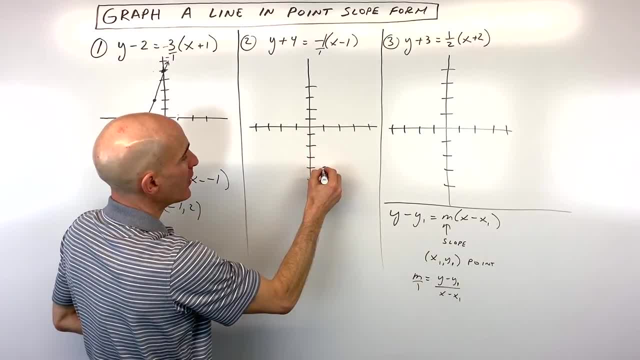 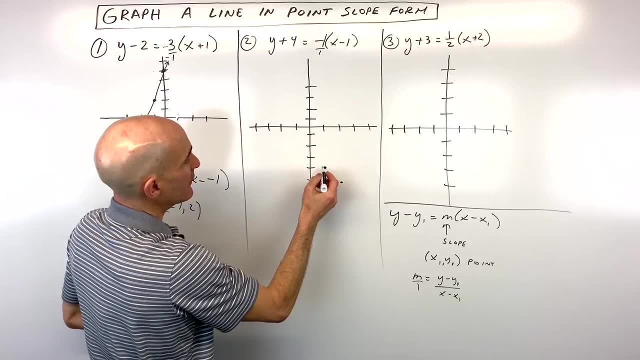 So write 1, down 4.. That's your point: that the line goes through And it has a slope of negative 1.. So we're going to go down 1, right 1. And if you want, you can reverse that. 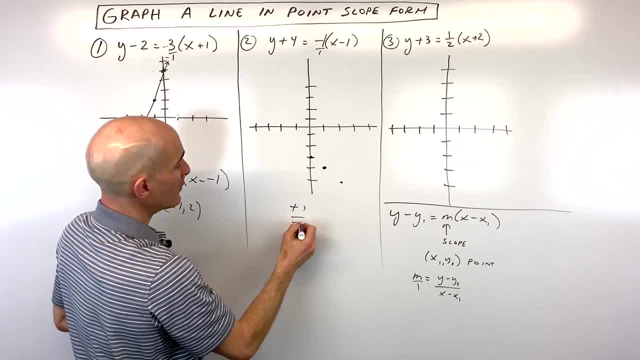 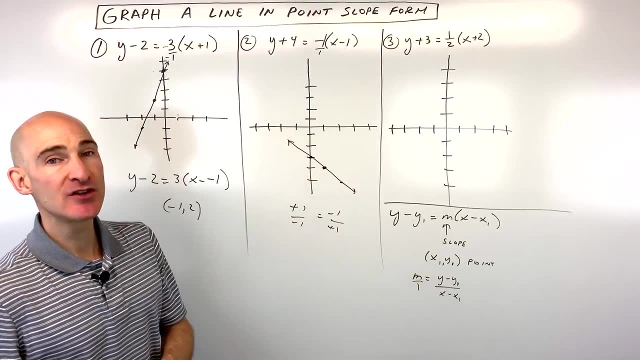 You can go up 1 and left 1, because positive 1 over negative 1 is the same as negative 1 over positive 1.. And so you can see there's going to be your line right there. Okay, last example: See if you can do this one on your own. 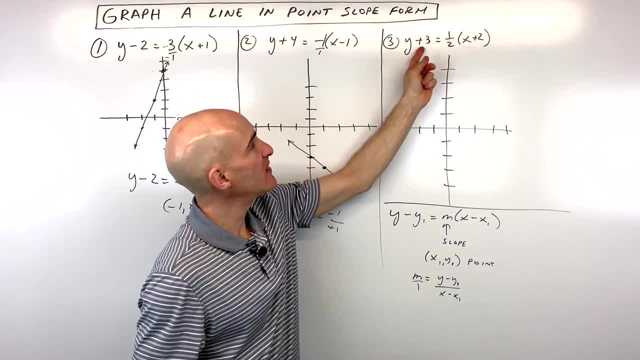 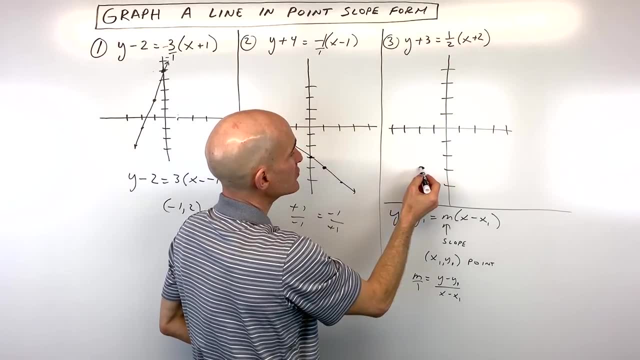 What point does this line go through? Negative 2, negative 3.. Remember, it's the opposite: Left 2, down 3, right about there It has a slope of 1 half. So we're going to go right.